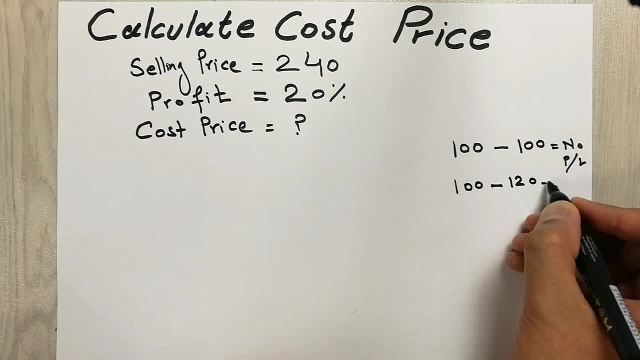 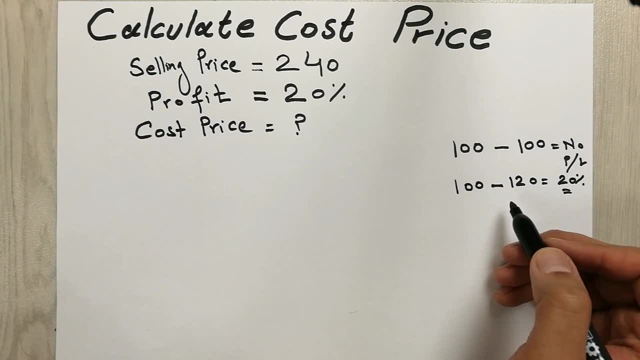 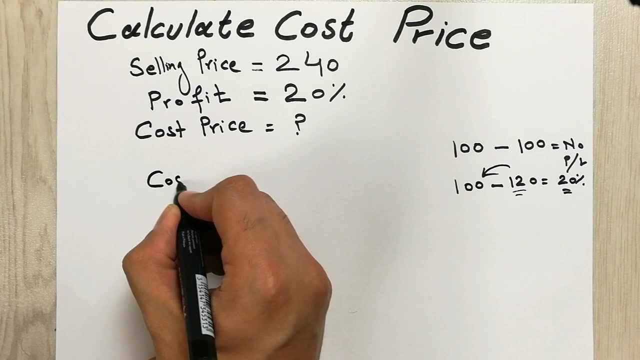 at 120, it means you made 20% profit. okay, so it means you sell that product at 120 percent of the cost price. okay, guys, so now what we will do. we will put the formula to find out the cost price. so cost price is equal to selling price. 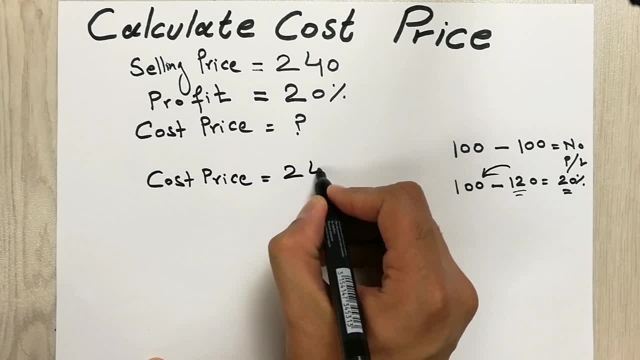 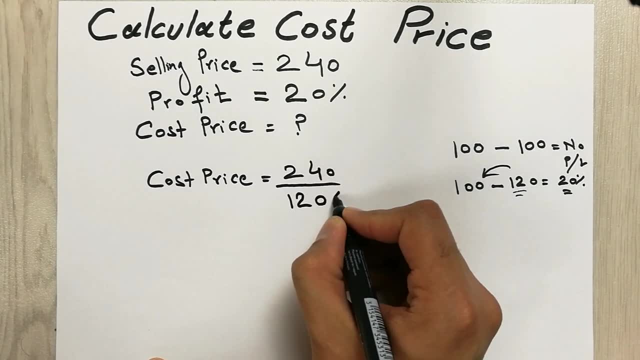 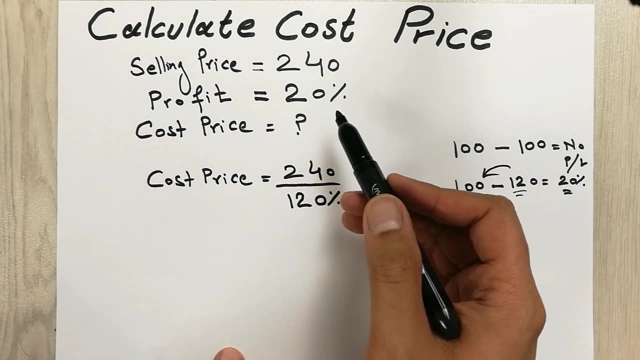 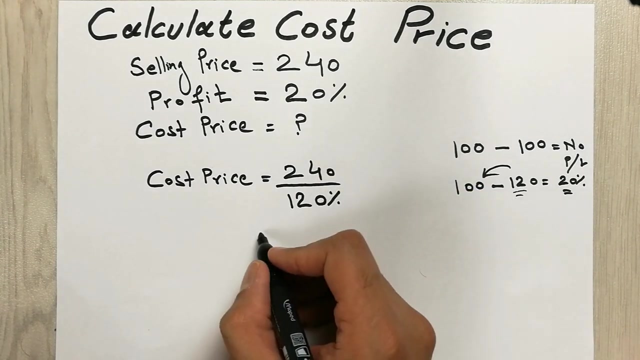 which is 240, okay, divided with 120 percent. okay, guys, because I already told you, because you sell it at 20 percent, it means you sell that product at 120 percent of the cost price. now we will simplify it. so 240 divided with 120. 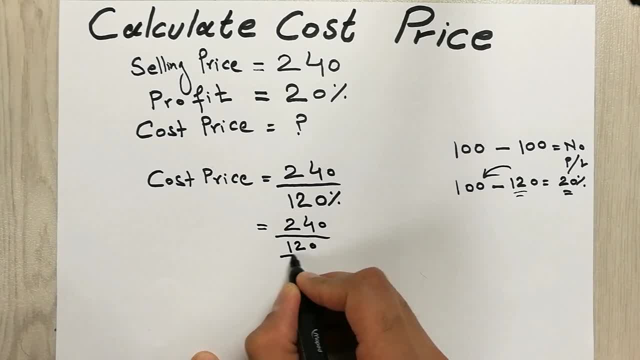 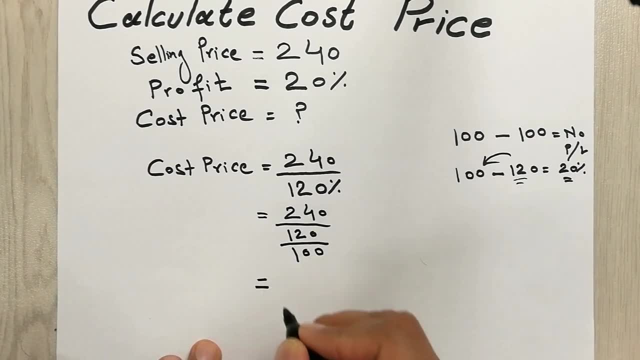 percent. it means 120 divided with 100. okay, guys, then in the next step, what we will do is: so 240, we will put it like that, okay, and this steps: 120 divided by 100, the answer will be one point two, okay. and then when we divide 240 with 1.2, 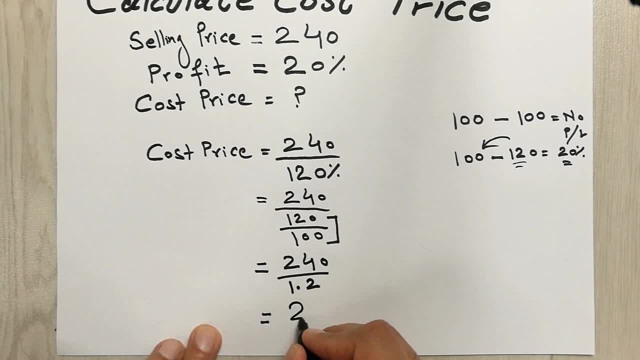 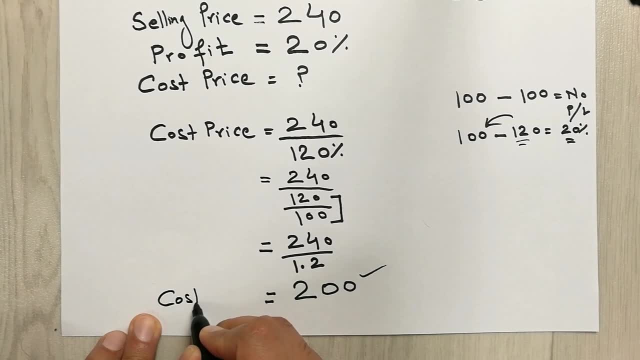 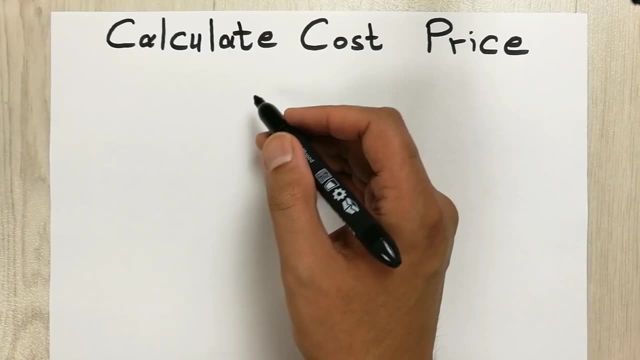 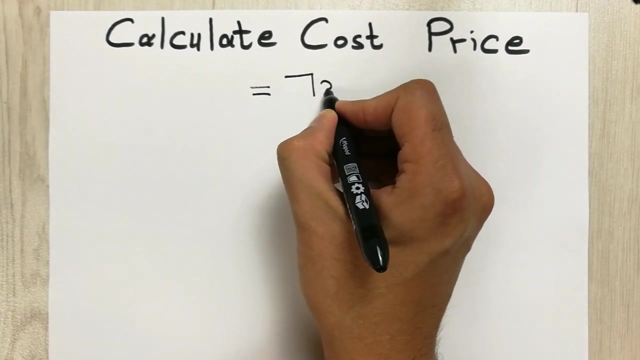 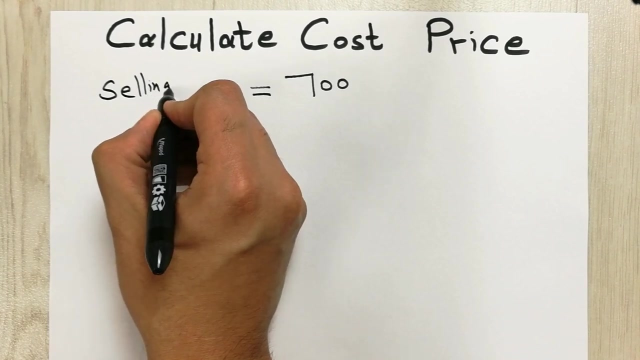 will be 200. so, guys, this is our cost price. I will show you with one more example. so, guys, let's say you have a product and you sold that product at 700 rupees or dollars. okay, so this will be the selling price. okay, and you made a. 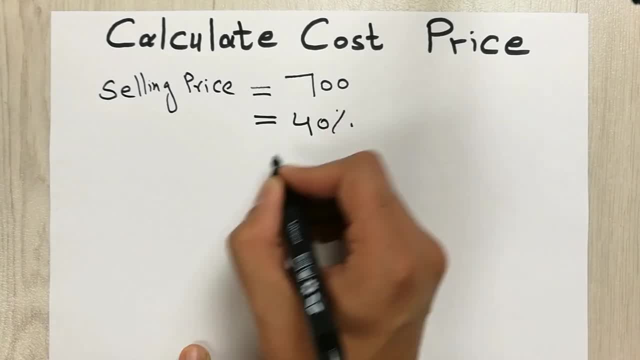 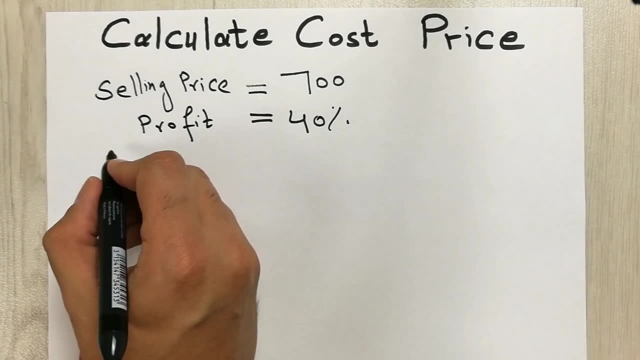 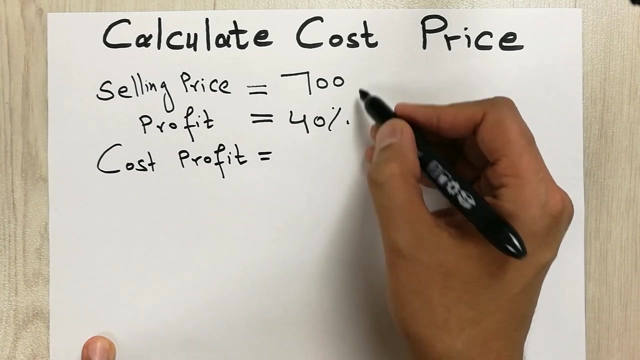 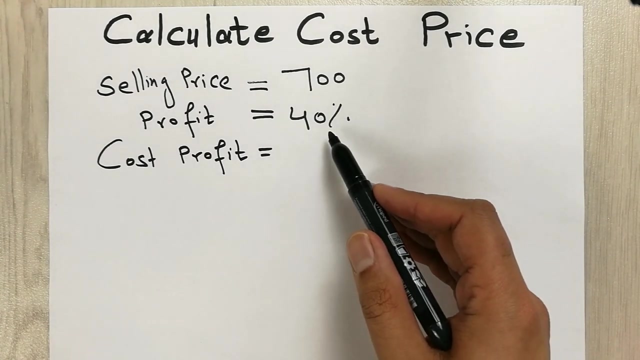 profit of 40%. okay, so this will be our profit. okay, and now you want to calculate what is the cost price, so how much that product costs to you. okay, when you have these two figures available. so now, as I told you before, the profit was 40%. it means you sold that item at 140 percent of the cost.